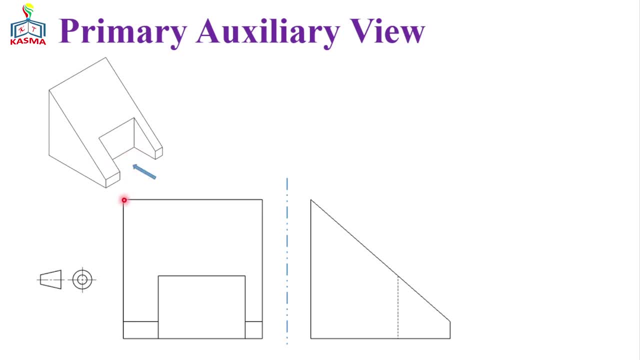 object is from this direction and then the left side views of the given object is from this one, and then it is constructed with the first angle projection system. So once we construct all the multi-viewed rings of this part, we can get this surface. The corner point to construct this inclined surface can. 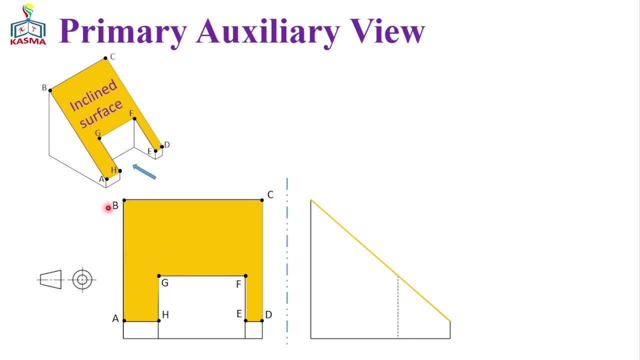 be labeled in this way. Thus, pointers will help us to transfer the dimensions of this surface into the exact surface. The views of this inclined surface from the front view can be sketched in this way, and it's a distorted surface. The exact shape of the surface is not. 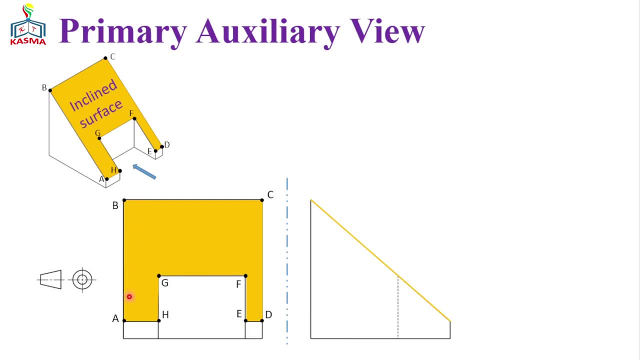 projected here And in the other one. if you look this one from the left side view, you can get an edge here. So this is just a line from here to here, and then all the pointers at the lower part, that means points A, H, E and D, will be just. 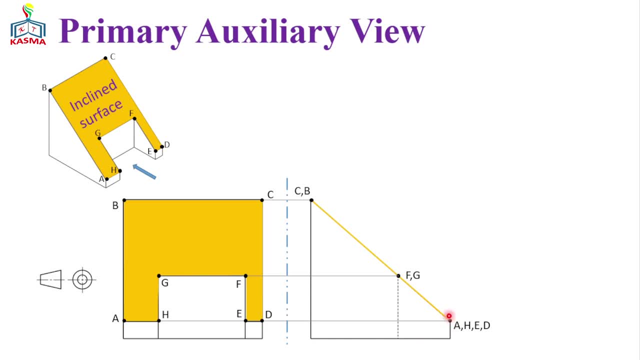 aligned at the same point, And in the middle one, G, F will be aligned over this one, and then B N, C will be aligned over this one, So the views of this inclined surface from the left side view will be just like this line. And then, finally, once we get all these, 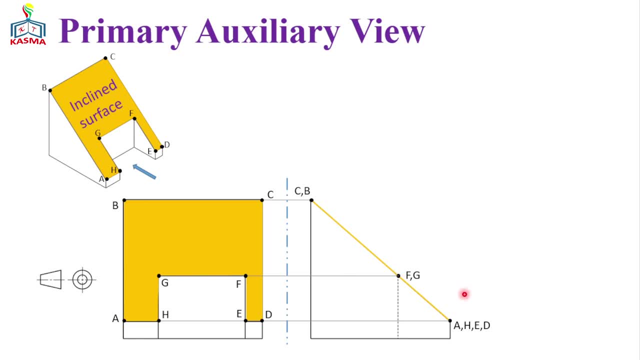 necessary pointers. we can project a perpendicular line from this slanted line. in this way, By considering the space we have to construct for a primary auxiliary view, we can draw the auxiliary plane line at a wished distance. The auxiliary plane line should be parallel to this edge view. We can measure the 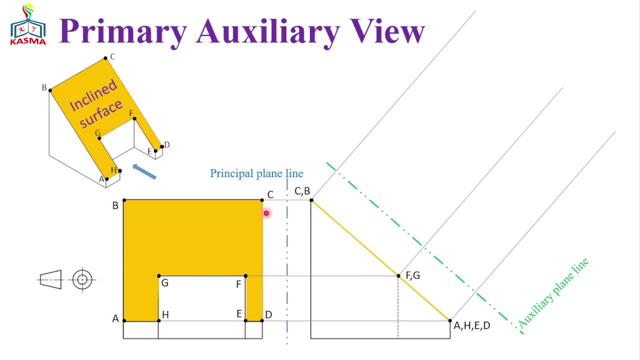 distance from the principal plane line to each point, and then we'll transfer that dimension with the reference of the auxiliary plane line. Now let's start from the lower part. We have four pointers, that is, points A, H, E and D on the lower. 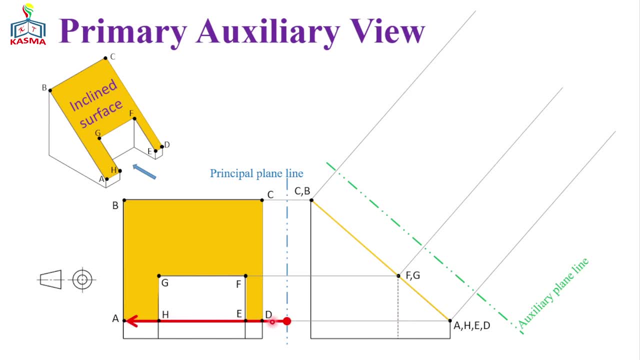 parts of this point. We can measure the distance from this reference plane line into these four pointers and we can transfer this dimension into this one from the references of the auxiliary plane line. And then, if you do that, since we have four pointers over here from here to here, 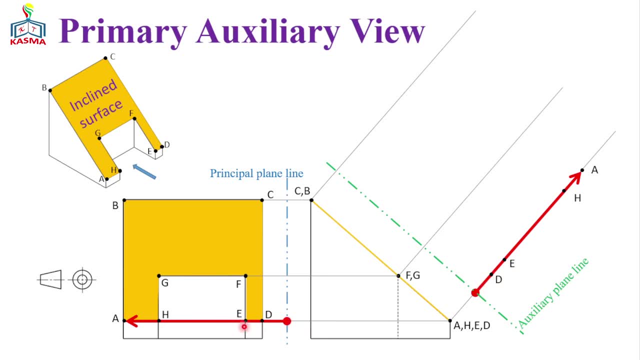 it will be point D, from here to here it will be point E, from here to here it will be point H, and then, from here to here, it will be point A, And then all the pointers can be scattered. in this way, We can measure the distance from this. 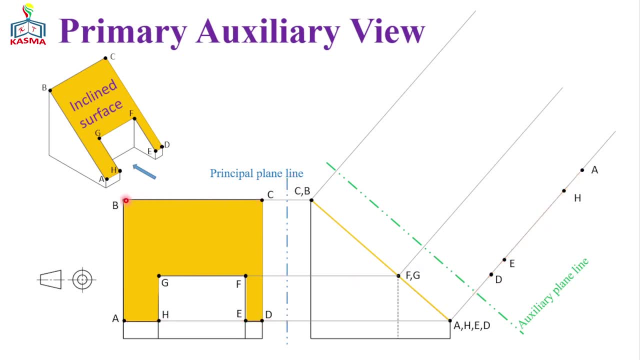 reference into the other pointers, that is, point B and point C. If you measure that, you can get this distance and then on this line you can measure all those pointers and then you can transfer that dimension and then, finally, point B and point C can be located over this specific location. 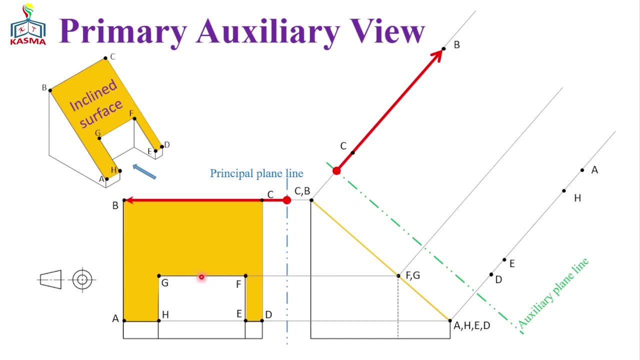 The remaining pointers are point F and point G. So you can refer this line and then you can measure from here to here and then you will get that dimension, and then you can transfer all those pointers and then finally you will get the exact positions of point G and point F, like this one. 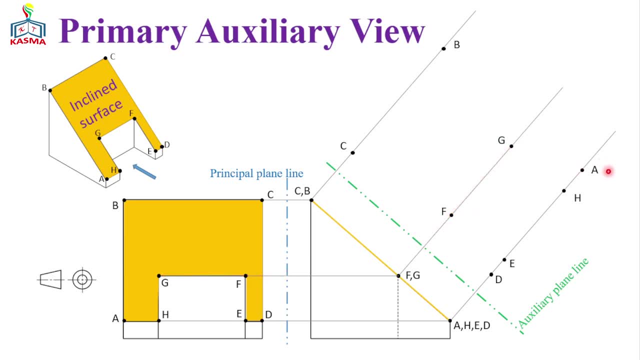 The last thing is we can connect all those pointers, starting from this point, Starting from the initial corner point, and this way, that means from point A, B, C, D, E, F, G and H, just like this one, And then the last one is from H and to A. 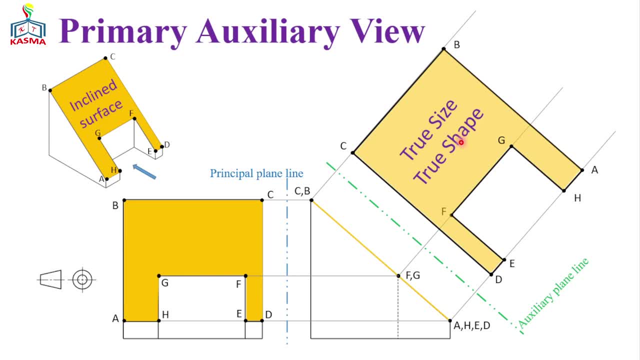 Finally, we can get this auxiliary view. So this auxiliary view is just with a true size and a true shape. So we can find out that inclined surface with a true size and a true shape. It will help us to give the dimensioning or to know the exact. 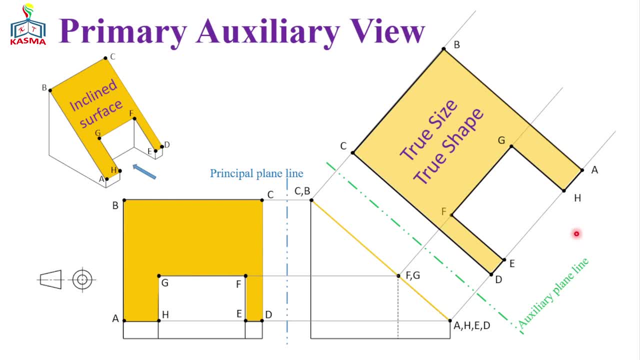 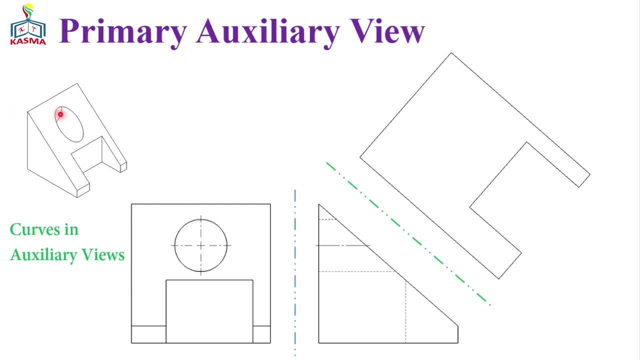 size of the given point. Now let's add one future here. The future is just the bore of this surface. So if we bore this one with a circular feature like this one, finally we'll have this object. So this object will have a crevice in the auxiliary view. 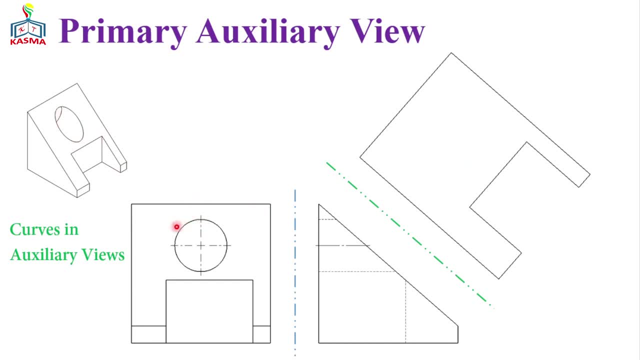 To contract such crevice on the auxiliary view. we can use the division method here, So we'll divide this circle on one view and then we'll try to transfer it into the auxiliary view. If you look here, this is just the circular feature on the front view and then this one will be on the left side view. 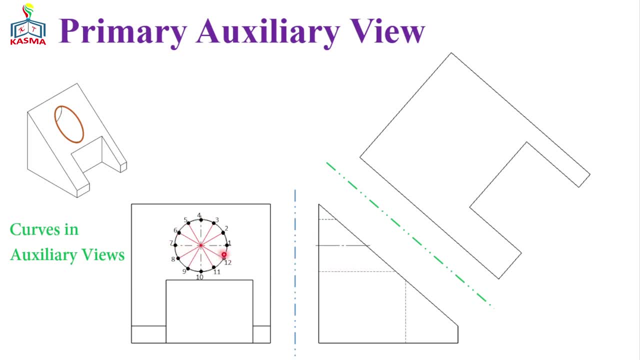 So the circular feature is on this portion, on the left side view, from here to here, which is represented with a hidden line. Now let's divide this circle into the number of sectors. If the number of sectors increase, then the accuracy of the represented view will be increased. And then, if you divide, 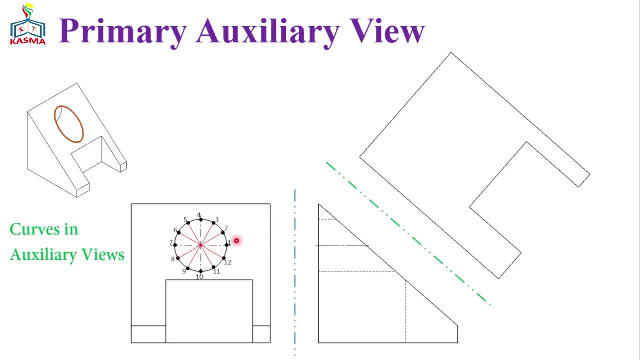 this into less, then the representations of the surface on the auxiliary part will not be as exact as expected. So let's divide this one into 12 parts. So if we want to divide it into 12, that means 360 by 12 will be a 30 degree. 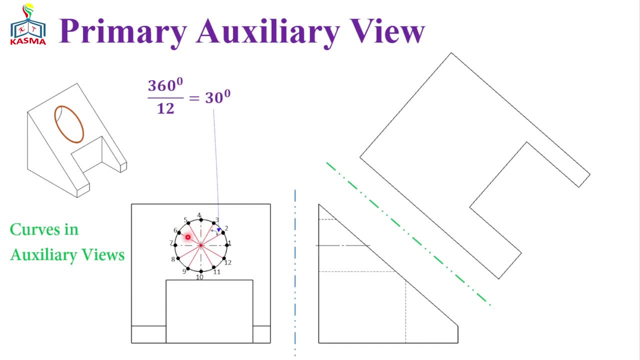 So each sector will have a 30 degree measurement and then their divisions will be in this way. So we just divided these parts into equal sectors. Now we can draw a construction line from each point to the inclined surfaces of the view like this one. 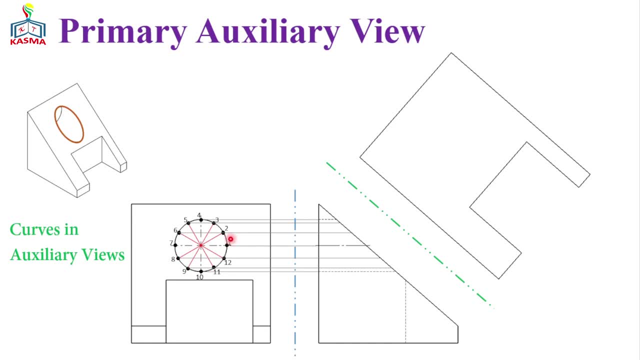 So from here to here, we'll just transfer all pointers, In this case points 3 and 5, 2 and 6, 1 and 7,, 12 and 8, 9 and 11 are just on the same line. 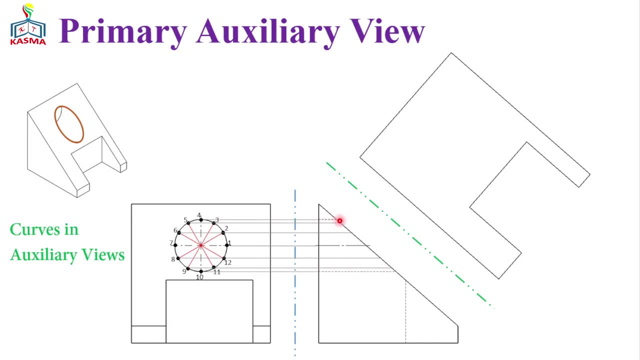 And then, once we do this, we can draw a construction lines which are perpendicular to this edge and then extended from these lines, just like this one. Then the same procedure can be applied: From the reference one we can measure the distance between this vertical reference line up to the points of the division. 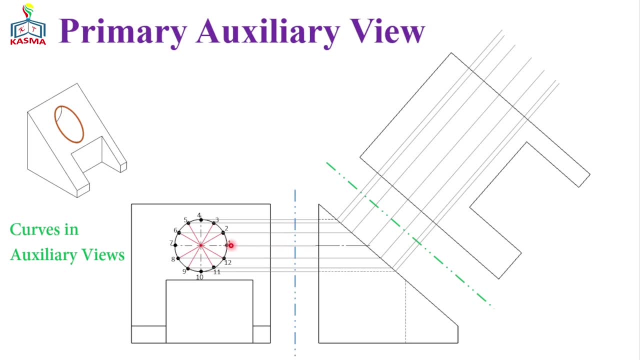 So, from here to here, if you measure this one, you'll get point 1, and then, from here to here, you'll get the measurements of point 2.. From here to here, you'll get the measurements of point 3, and then, from here to here, it will. 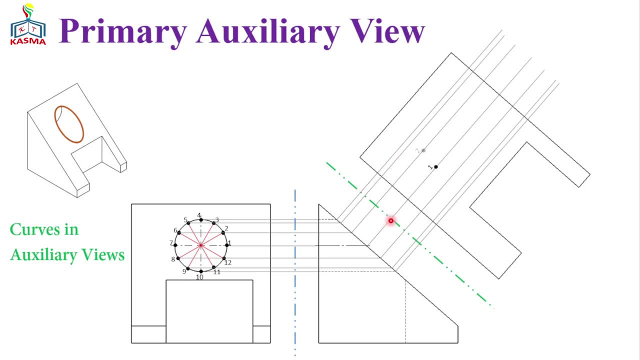 be the measurements of point 4 etc. Once we measure all the dimensions of the pointers from the principal plane line- that means the first reference- and then transfer the dimension into the auxiliary plane by the auxiliary plane line, then finally we can get all the 12 pointers scattered in this. 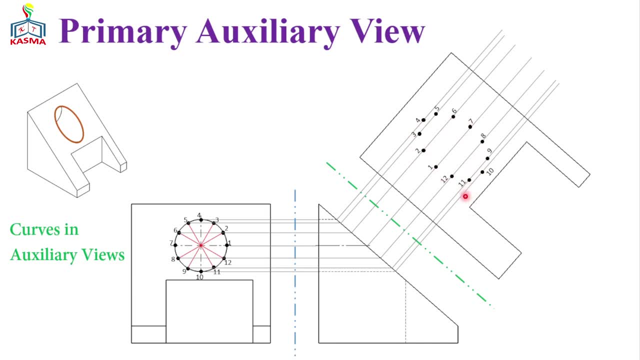 way, And then, once you get all those pointers, you can use a French curve to connect them, and then, by using a French curve, you can just connect them and then finally, you'll have such types of elliptical curve. Let's see a practical example here. 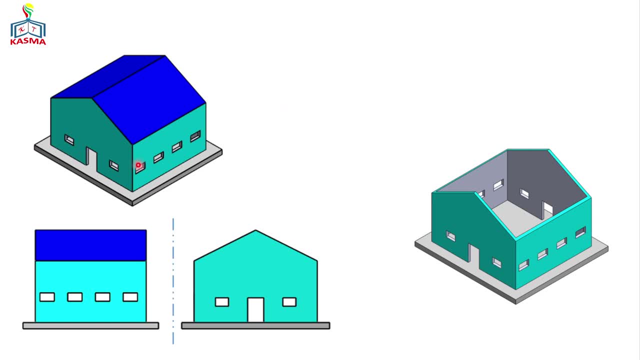 For example, if there is a house just like this one and then if you look this house from the front view, you will have this surface, and then from the right side view, it will have this surface. If you look the views of the roof, it is just distorted on the right side view. 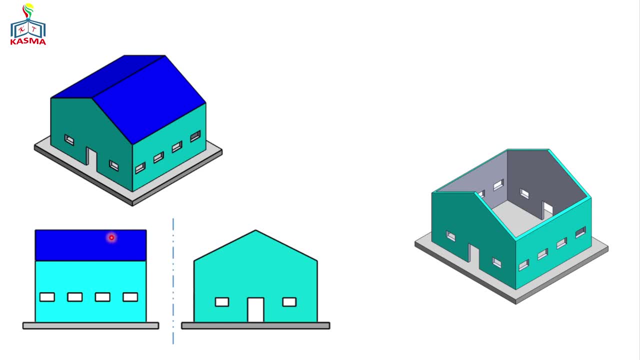 So how we can get the exact sizes of this roof? If we just use the roof as of the views here, it will have such types of cover or the roof will be this one. So we have to use the auxiliary view to know the exact size and shape of the roof.